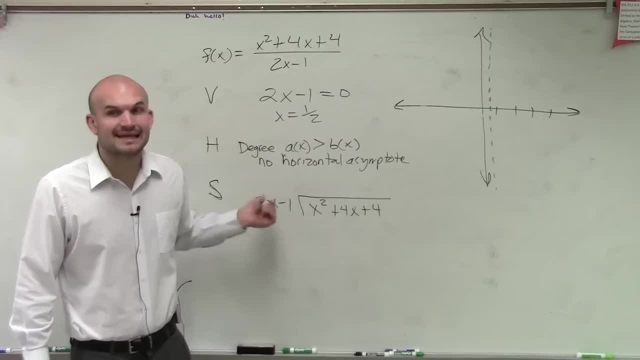 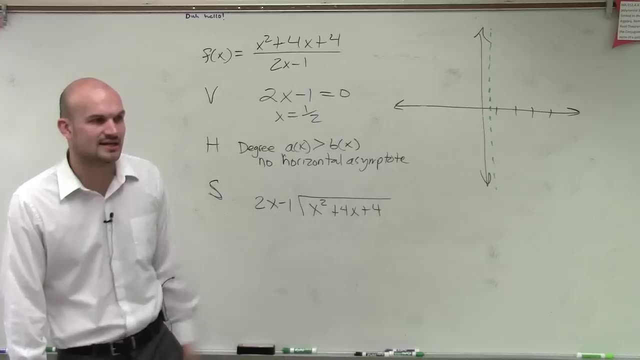 is when your divisor is a linear binomial. Well, this one is linear because it's x raised to the first power and it is a binomial. So we could use synthetic division, but let's get a little practice with long division. 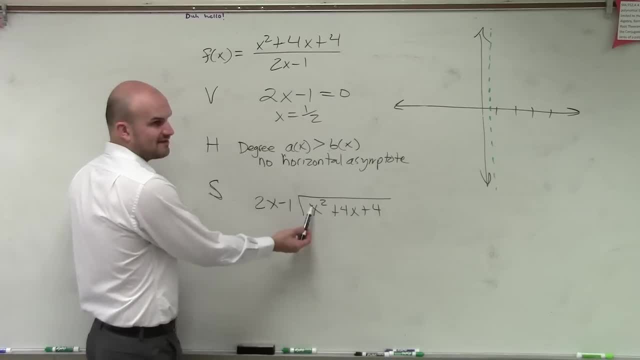 So we say 2x divides into x, squared. Well, 2 divides into 1, 1 half x divides into x, squared x times. Now let's double check to make sure that works. Now, remember, once you have this: 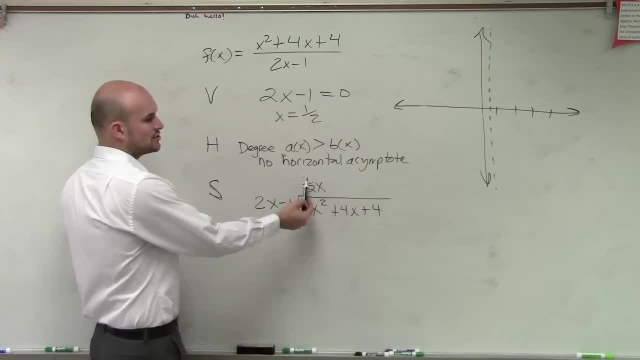 you've got to multiply this term times both of your divisors. So 1 half times x is x squared. Remember, whenever you multiply this number back, you have to get that same term. OK, Eva? Then I do 1 half times x, which is going to be a negative 1 half. 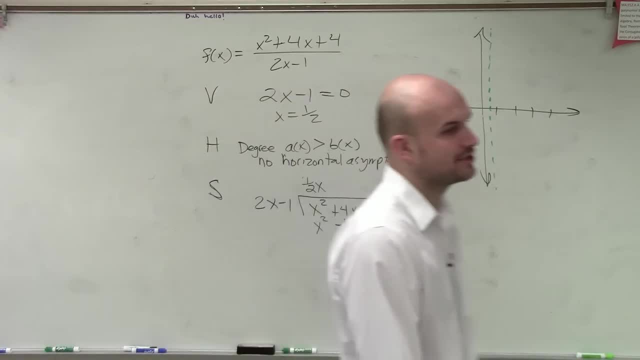 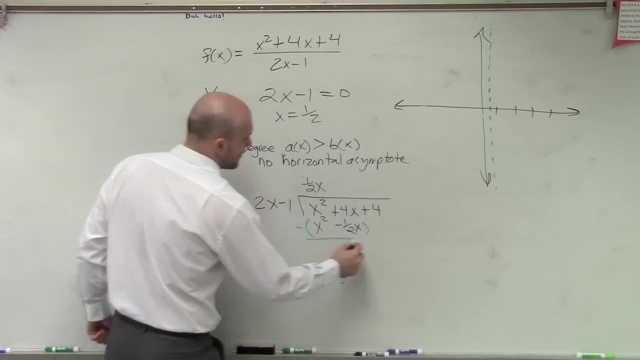 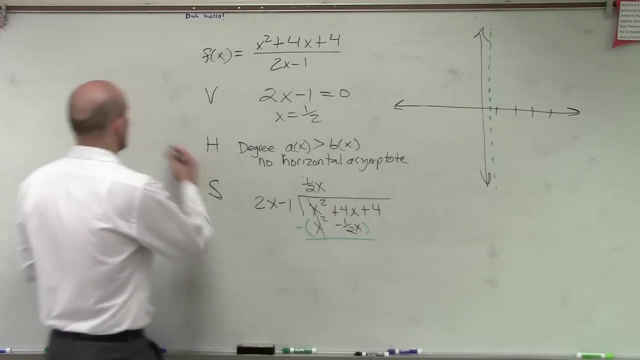 x. Now the next thing we do, if you guys remember, we have to subtract the whole row. So x squared minus x squared is just 0x squared right, So that always goes to 0.. But now I have 4x minus 1 half x. 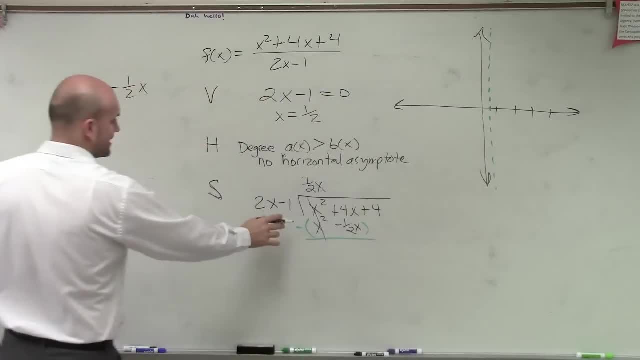 You've got to have them be the same denominators, right? I'm sorry, That is no, it's plus, It's minus, a negative, right? So now I need to add these up. So therefore, instead of 4, I need. 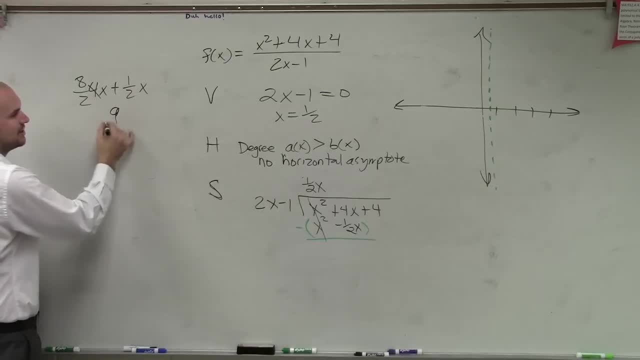 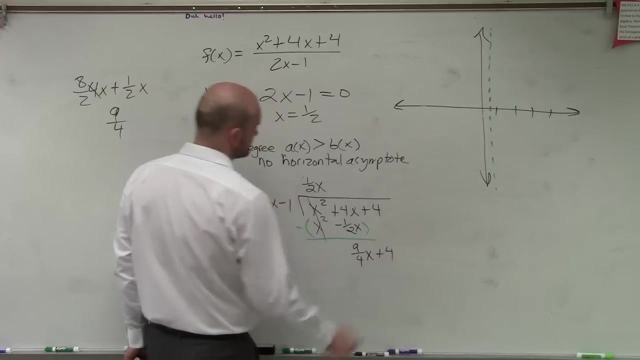 to rewrite this as 8 over 2.. So this is really 9, 4x. Yes, Yes, Yeah, Good. So therefore 4x plus 1 half is going to be 9 over 4x and then plus 4.. 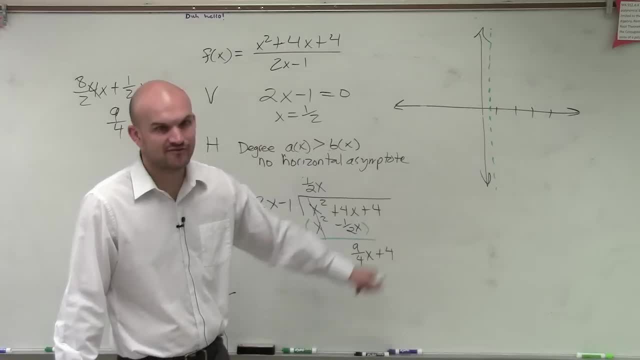 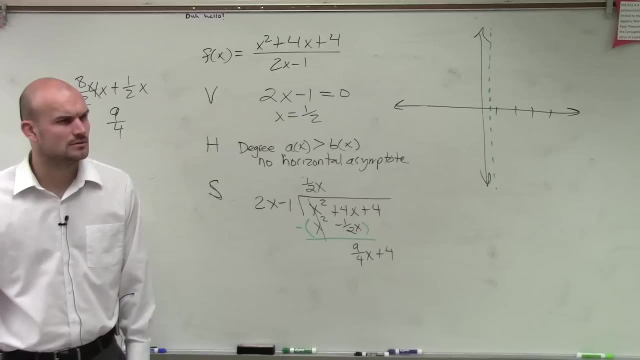 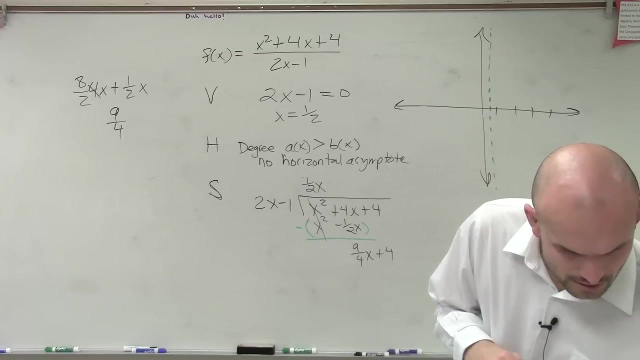 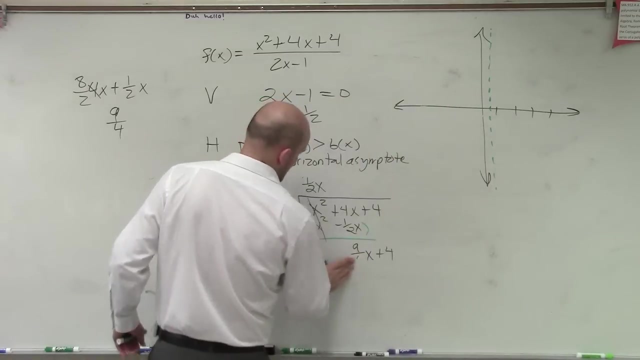 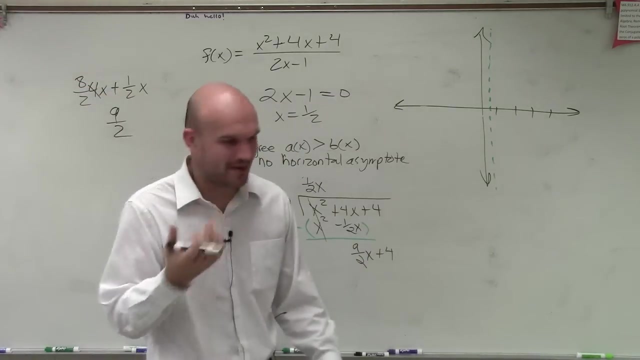 So now we say 2x divides into 9 fourths. You have what? Oh, what am I doing? That's 9 halves. What am I doing? Why am I adding it to 4?? I was thinking because I was looking back at my problem. 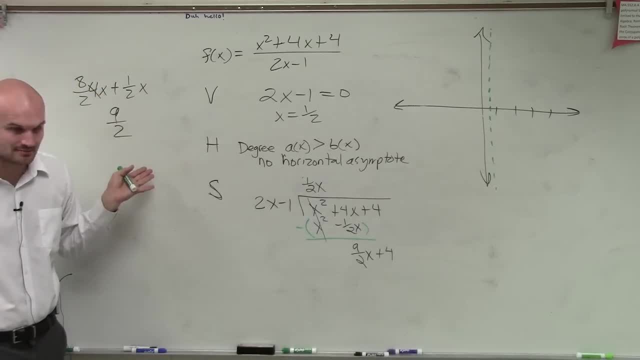 It's 9 halves, all right. It's 9 over 2, correct? Okay. so 2 divides into this how many times 9 over 4.. Let's check our math. How do we know if that's correct? 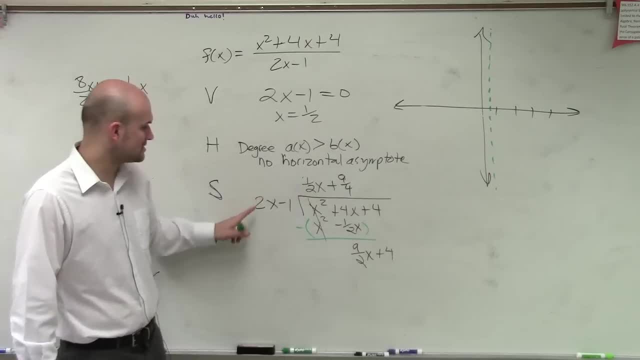 Remember: you multiply 9 fourths times 2x 9. fourths times 2x 9 fourths is 9 halves x 9 fourths times negative 1 is a negative 9 over 1.. Then you subtract the rows. 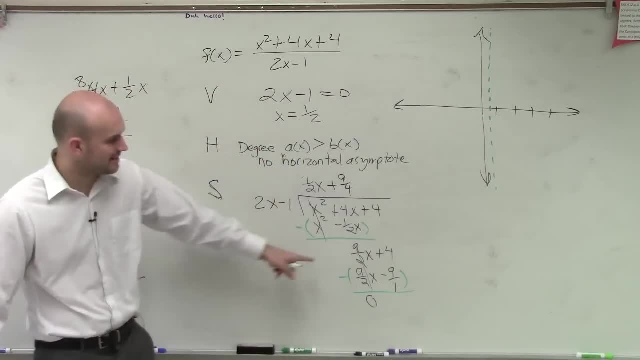 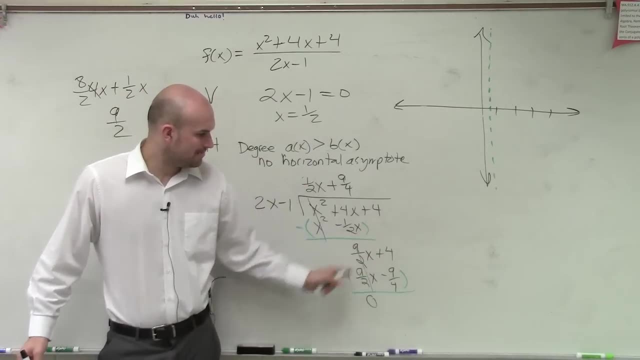 This again goes to 0.. And then, ladies and gentlemen, you could do 4 minus a negative 9 fourths. But, ladies and gentlemen, isn't x going to divide into that? No, It's not going to divide into that number anyways. 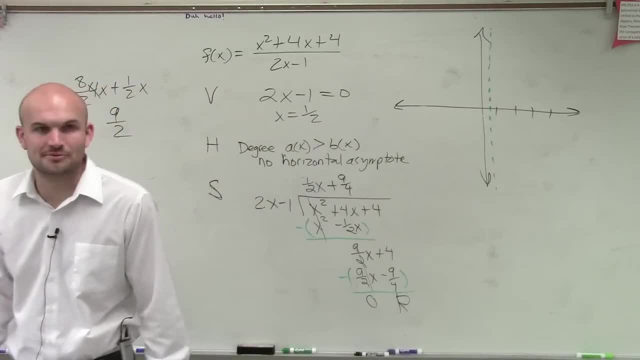 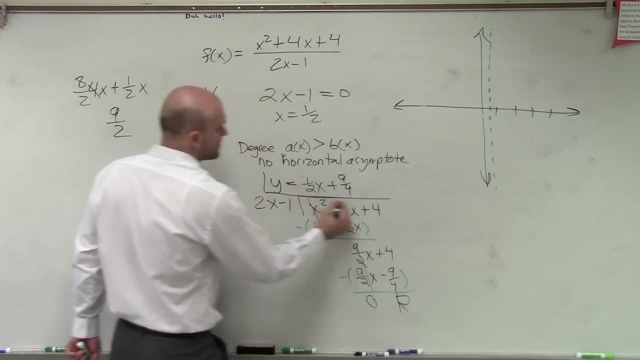 No. So guess what? That's your remainder. And I said slant asymptotes. Do you deal with the remainders? No, So therefore our equation for our slant asymptote is: y equals our quotient. So now we need to graph that. 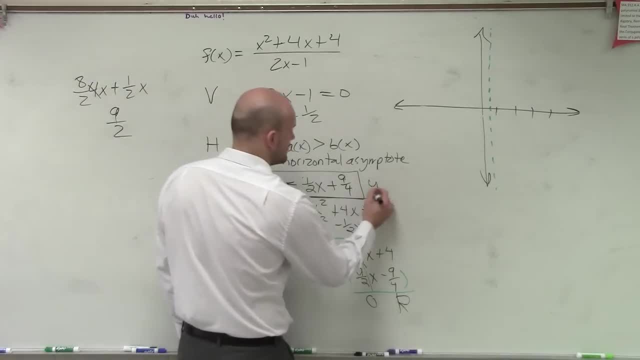 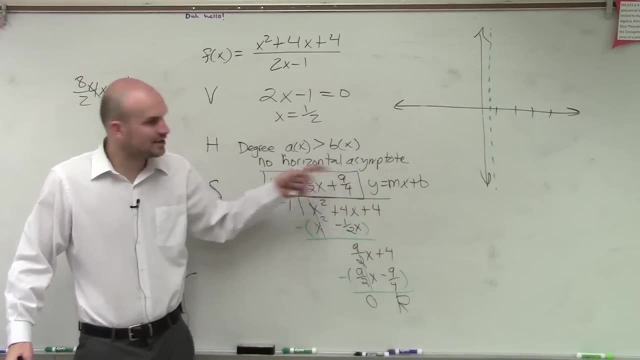 All right. So how are you going to graph that? Well, remember all linear equations we can write in: y equals mx plus b form, where b is my y intercept. So the y intercept is at 9 fourths, Which is 2.25.. 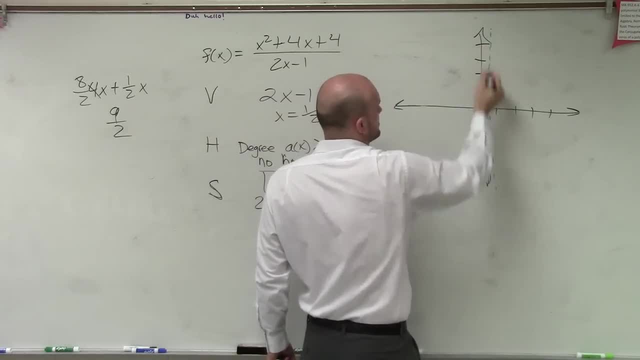 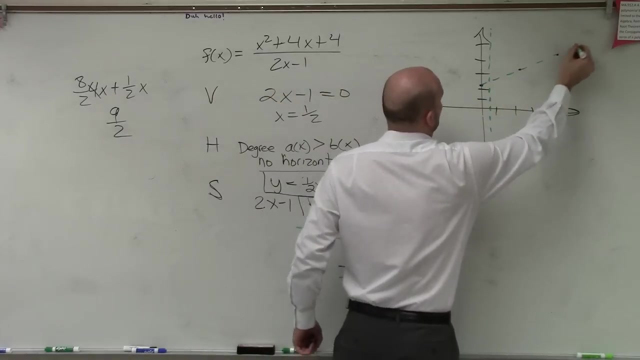 So let's just go up to 2.. 2.25 is going to be roughly around there, And then we're going up 1 over 2.. Up 1 over 2.. Up 1 over 2.. So we're roughly going to have a graph or an asymptote. that's. 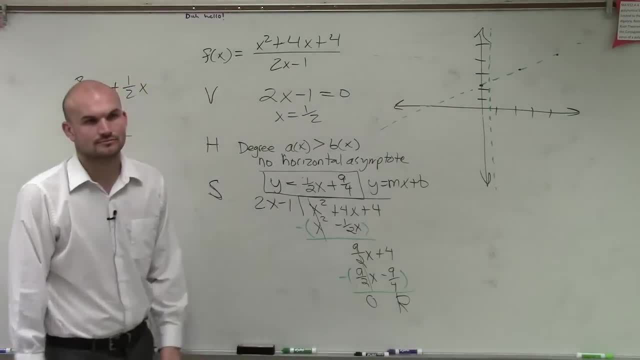 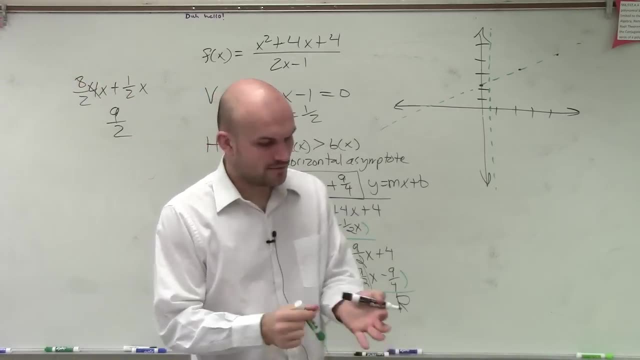 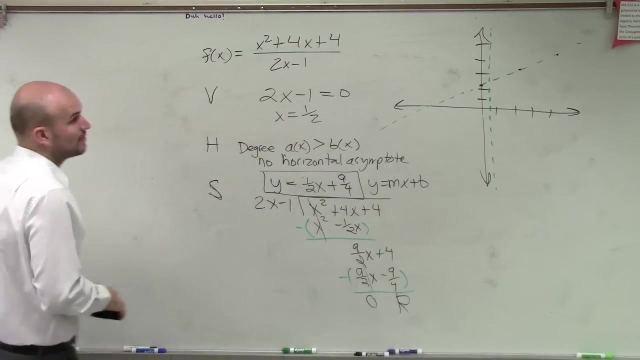 going to follow that line. Does everybody see what I did with that? Yes, Kind of Yes, No, Maybe. so All right. So now we did the long division to find our slant asymptote. Now what we're simply going to do is still we 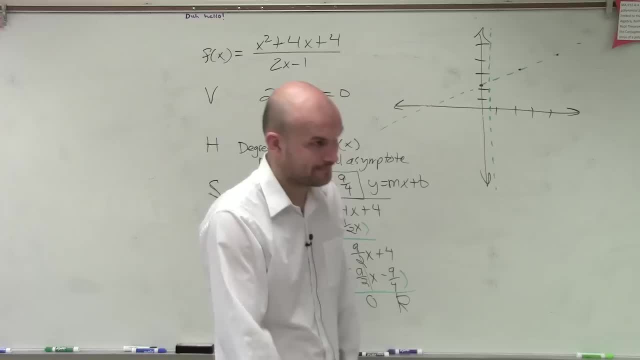 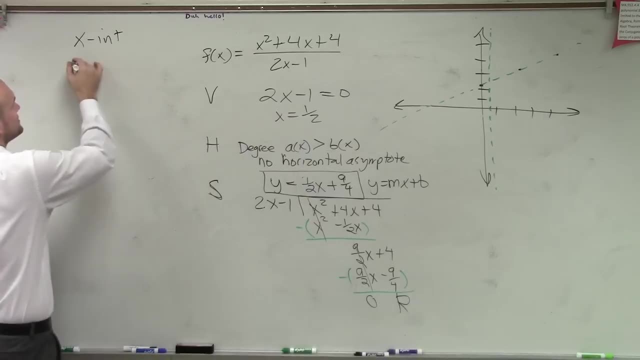 need to find our x and y intercepts. All right, So let's do the x intercept. x intercept is when y equals 0.. 0 equals x squared plus 4x plus 4 divided by 2x minus 1.. 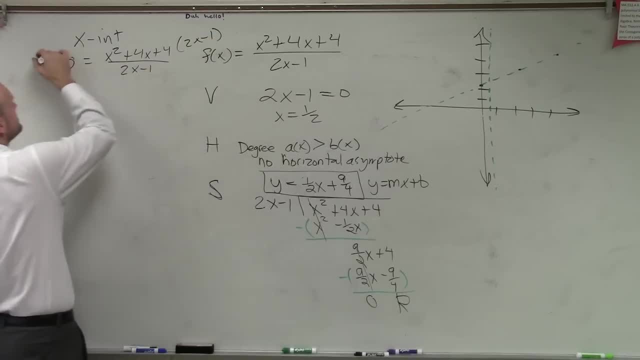 Here. we need to get this off the bottom. So we multiply 2x minus 1.. We multiply 2x minus 1 on both sides, That goes to 0. That divides out to 1.. So 0 equals x squared plus 4x plus 4.. 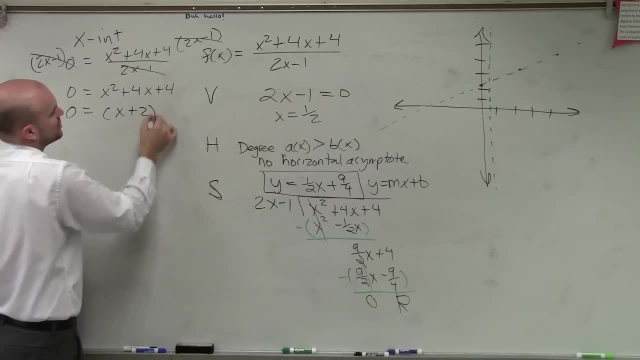 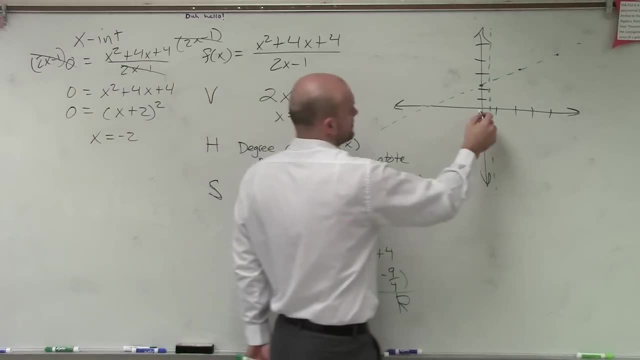 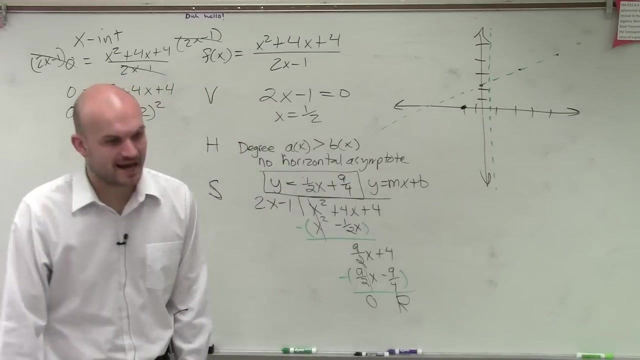 We can solve this one by factoring: 0 equals x plus 2. squared x equals negative 2.. Yes, So we could say at negative 2, we have an asymptote. Yes, Yes, Yes, Yes. What do you want to do? 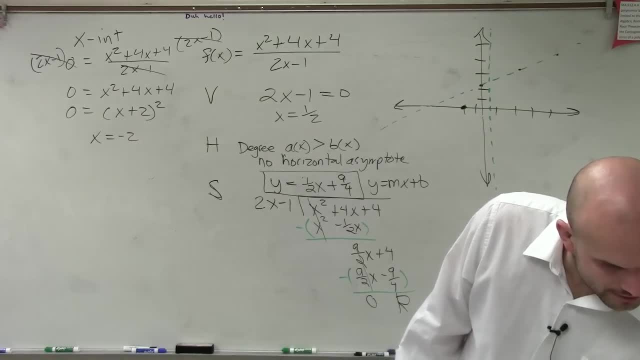 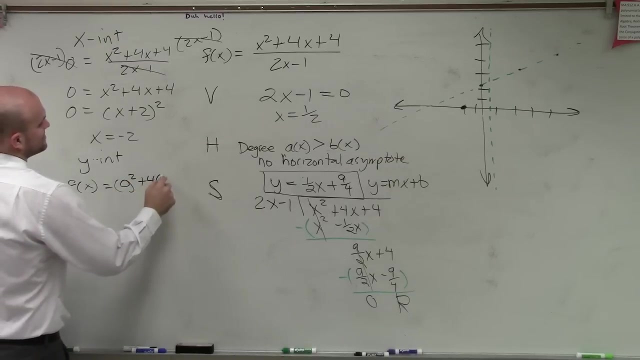 I'm doing 3.. OK, And then we need to find our y-intercept. So y-intercept is going to be: f of x equals 0 squared plus 4 times 0 plus 4 divided by 2 times 0 minus 1.. 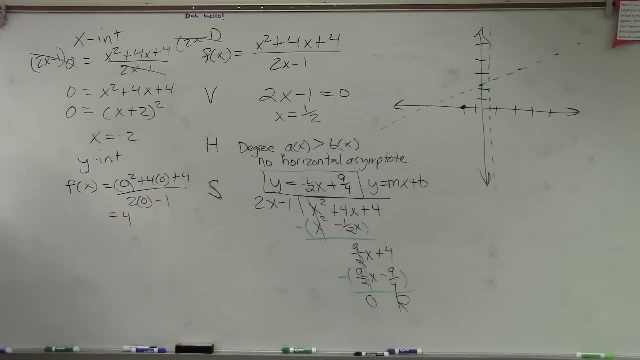 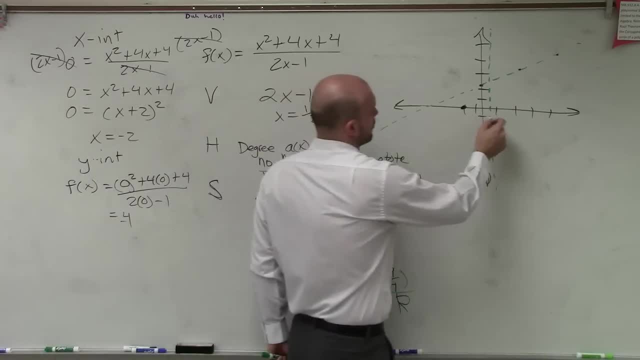 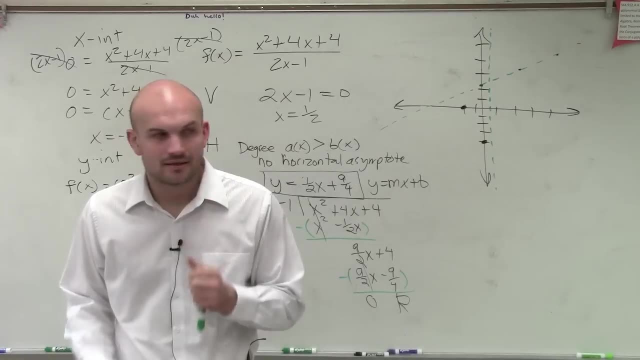 so it's negative four, right, So now we go: one, two, three, four. Okay, now let's go and take a look at this, guys. all right, If we're going to graph this, we still have to pick two points to. 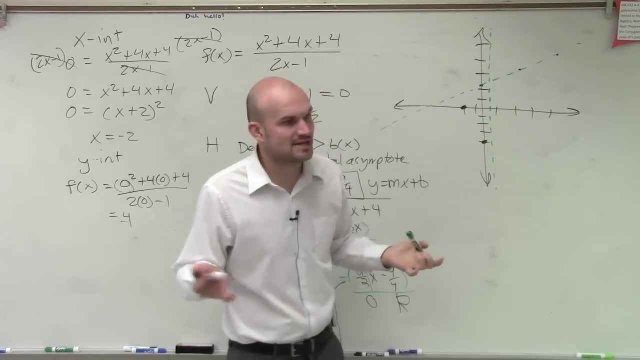 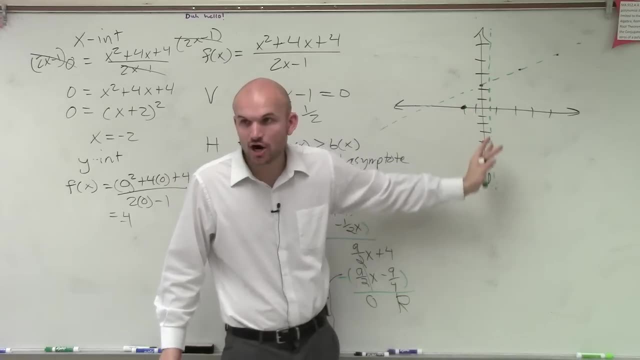 the right, which I'll go through in a second. But, ladies and gentlemen, remember we talked about our asymptotes. Our graph has to approach these two lines, right, It has to approach our horizontal, our vertical asymptote and it has to approach our horizontal asymptote. So for this, 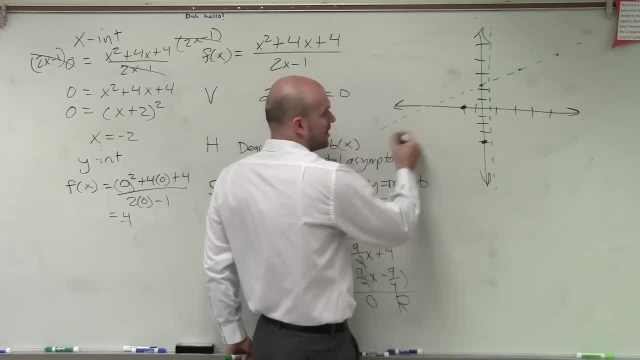 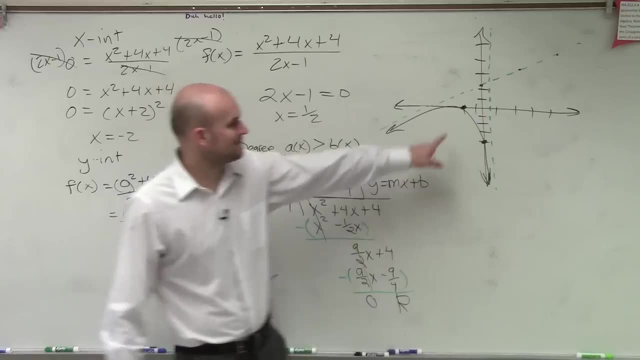 graph to approach, it has to go through these two points, all right, And then it's also going to have to approach these two lines. Now, how do I know? the graph only touches at this point and then rebounds. If you guys remember, it's not a whole big thing right now, but since 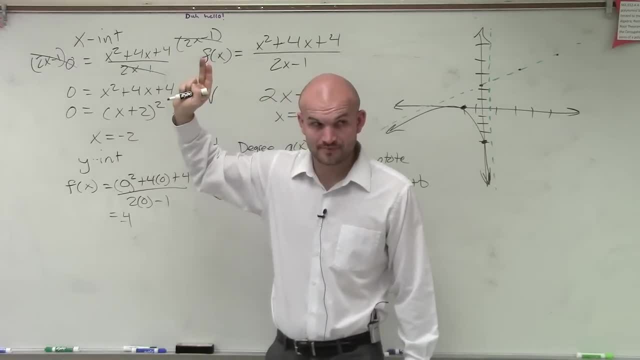 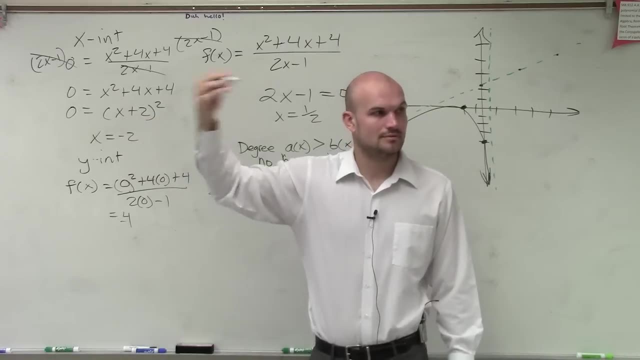 the graph only touches at this point and then rebounds. if you guys remember, it's not a whole big thing right now, but since this zero has a multiplicity of two- we talked about this in the last chapter- Since this has a multiplicity of two, it touches the graph but does not cross. So 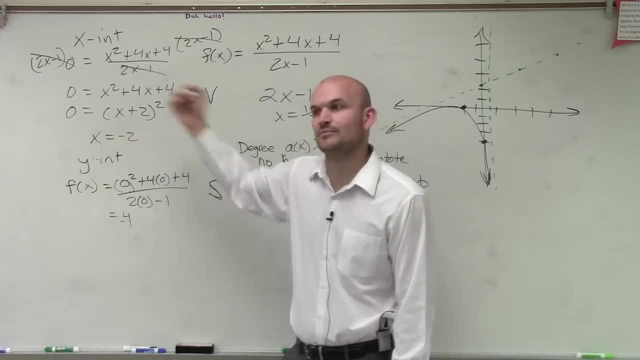 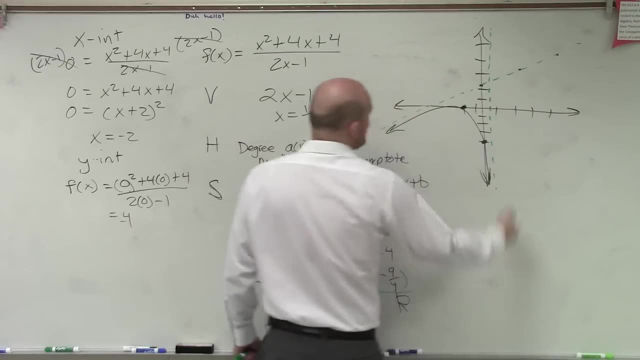 since it has an even multiplicity. it touches the graph but does not cross. So therefore, I know that it just touches and rebounds, but you guys, that's not our main focal point right now. Now, let's pick two points to the right. So let's do f of one. So, if I was to do f of one, 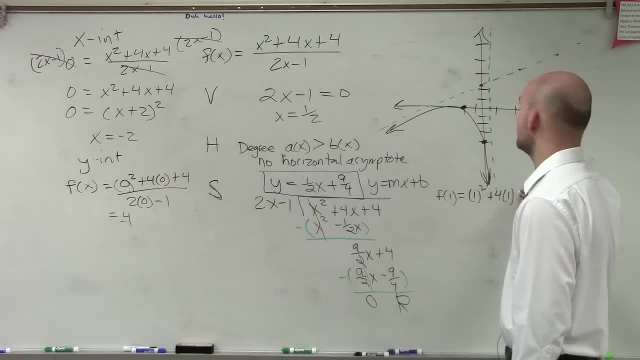 I do one squared plus four times one plus four, divided by two times one minus one. So we get one squared plus four is five plus four is nine, And then this becomes two times one is two, nine over one. So at one I go up to nine. One, two, three, four, five, six, seven, eight, nine, And then let's do f of two, So I do two squared plus four. 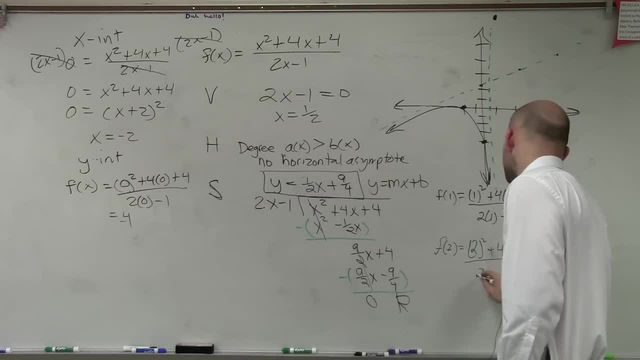 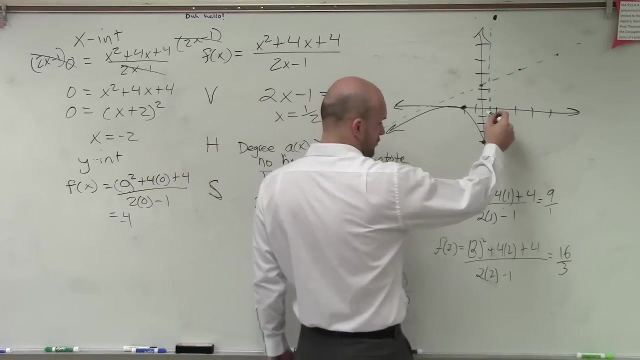 times two plus four, divided by two times two minus one, So this is four plus eight, which is 12, which equals 16.. Four, 16 divided by three is going to be five and one-third right, So we go over two. 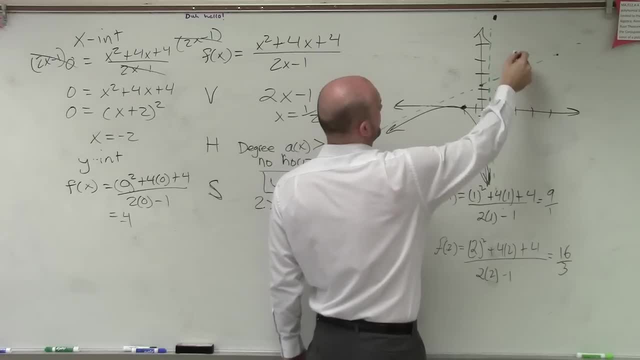 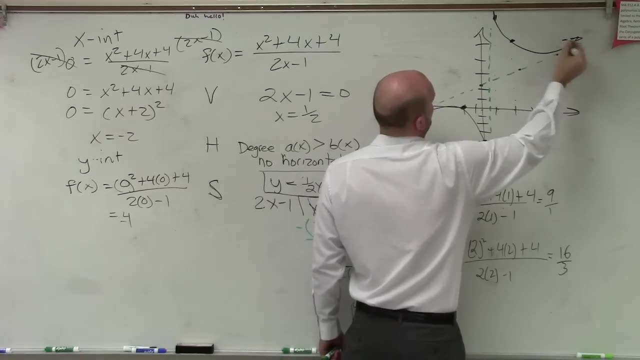 And we go up five and one-third: one, two, three, four, five And one-third. So what you guys are going to see is The graph is going to be somewhat of the same thing as my other graph, going right there. 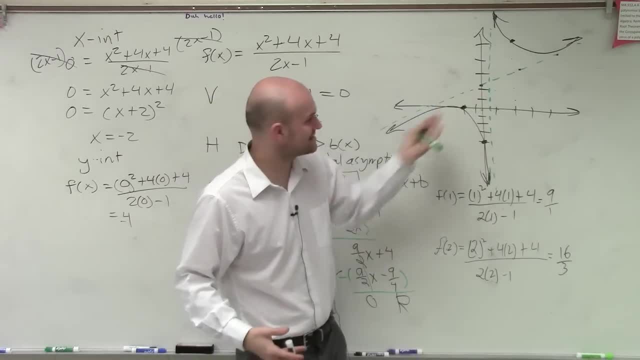 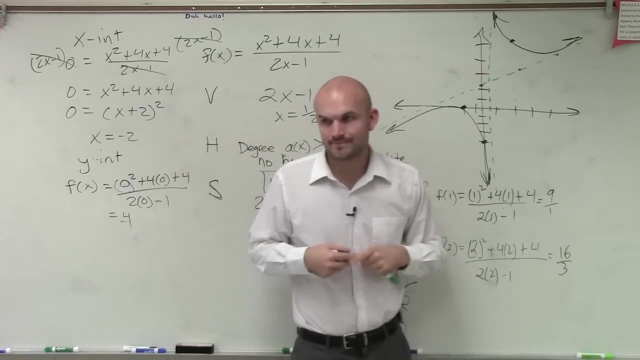 I know my graph's not perfect. You guys are going to have grid lines. I don't have grid lines, but you can see that these are like kind of the exact opposite, or the same graphs just in different parts. OK, So that is how you do a slant. 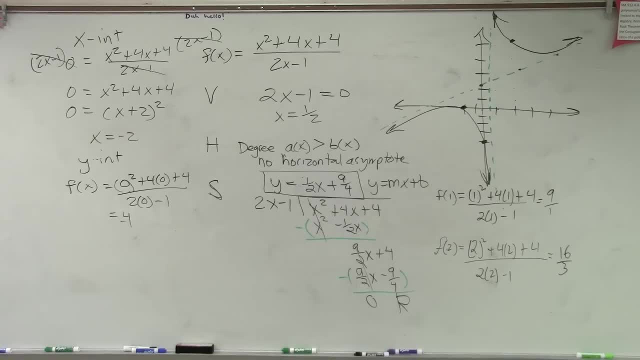 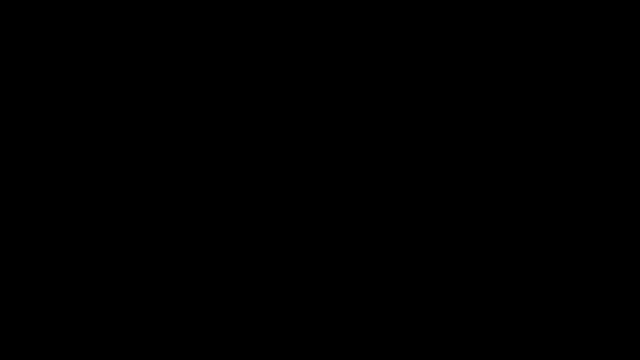 Yes, Sure, OK, I know these are long, long videos, so I'm just going to end it here.